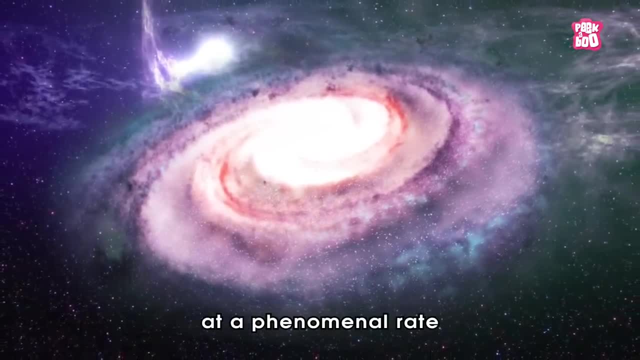 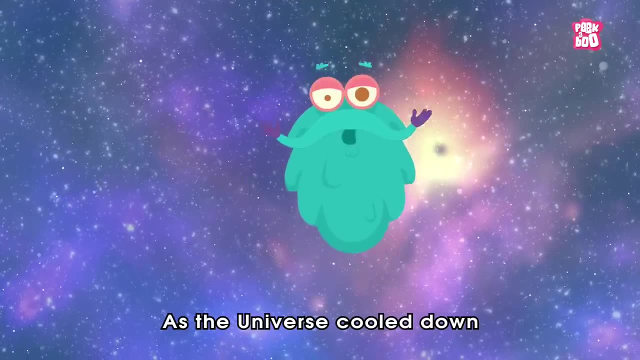 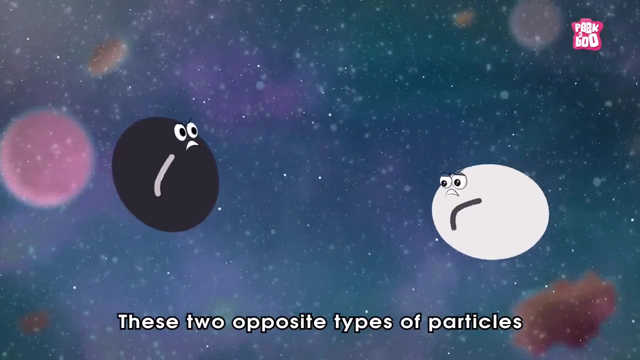 And it kept on expanding at a phenomenal rate And continues to grow even today. As the universe cooled down, the energy converted into particles of matter and antimatter. These two opposite types of particles fought hard and largely destroyed each other. 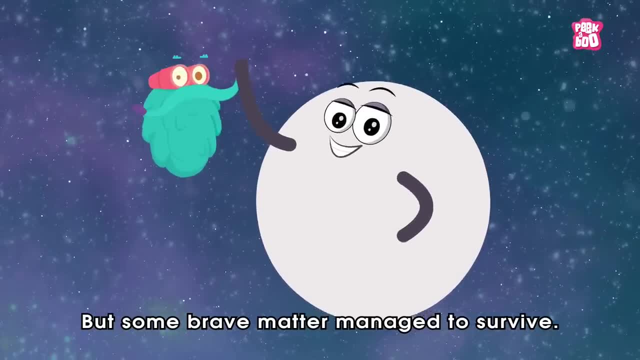 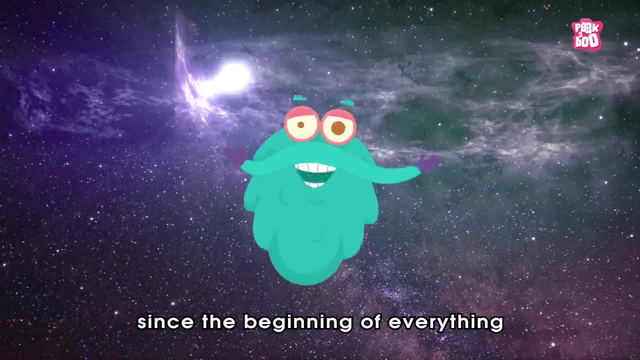 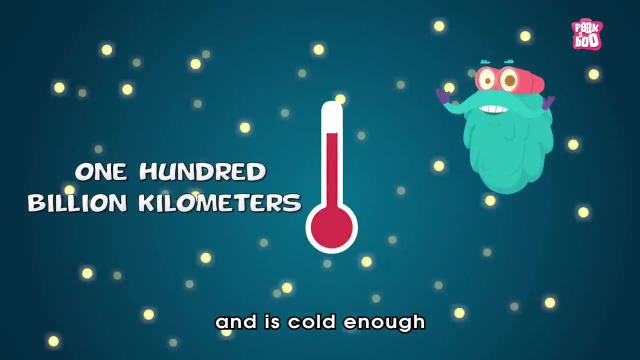 But some brave matter managed to survive. Please note that just one second has gone by so far since the beginning of everything, And the universe had already grown into 100 billion kilometers And is cold enough to form more stable particles called protons and neutrons. 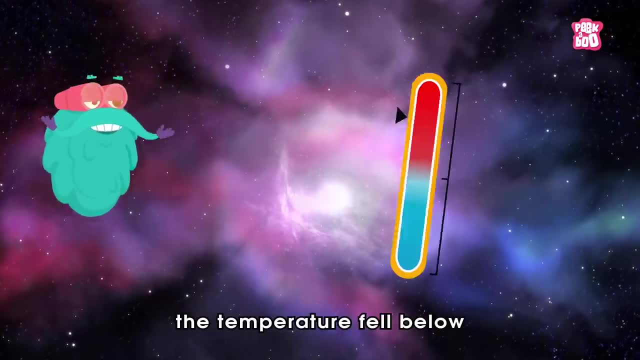 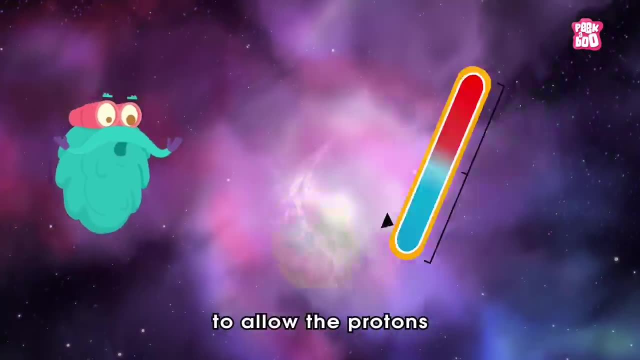 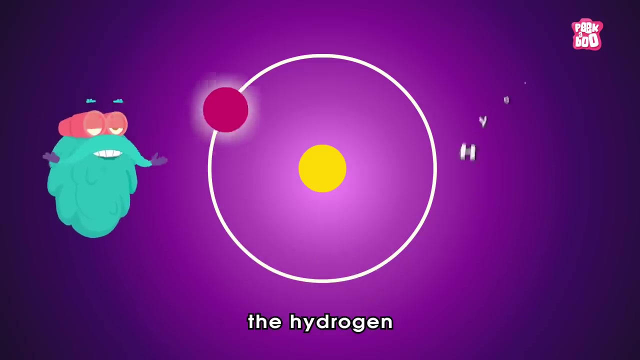 Over the next three minutes. the temperature fell below 1 billion degrees Celsius. Now the universe got more cold to allow the protons and neutrons to come together and form its first atom, the hydrogen. After millions of years, when the hydrogen gas clumped together, 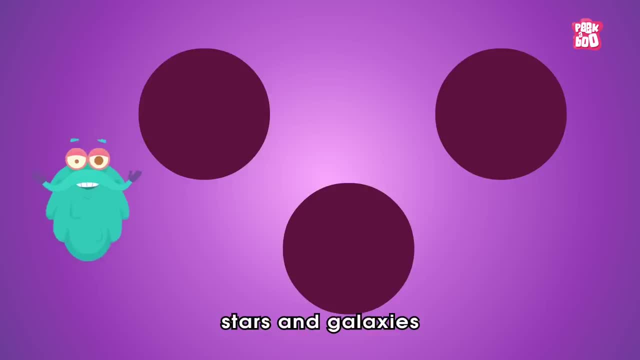 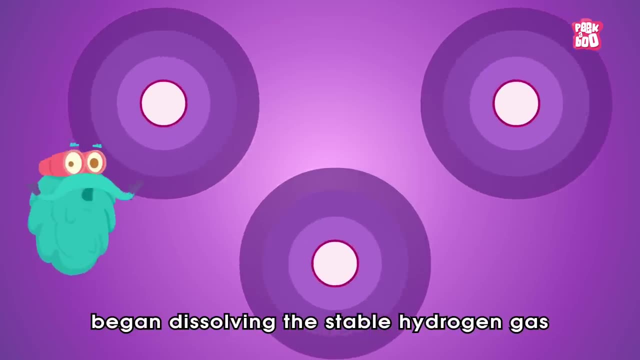 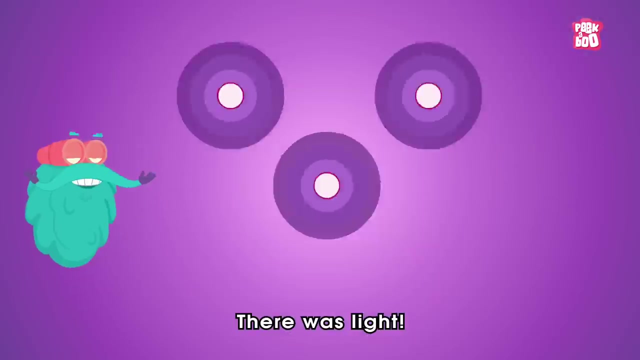 and gravity started to put it under pressure, stars and galaxies began to form Their radiation began dissolving the stable hydrogen gas into plasma that allowed visible light to pass, And finally, there was light Trivia time. Did you know? 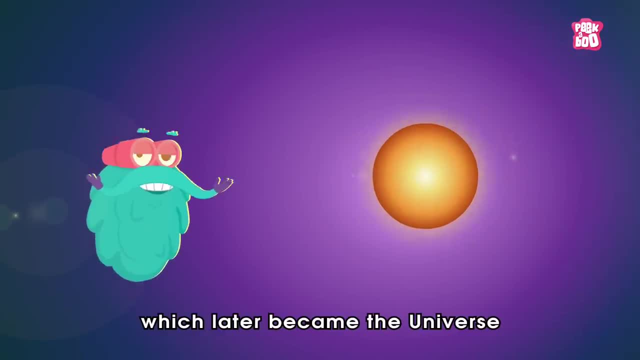 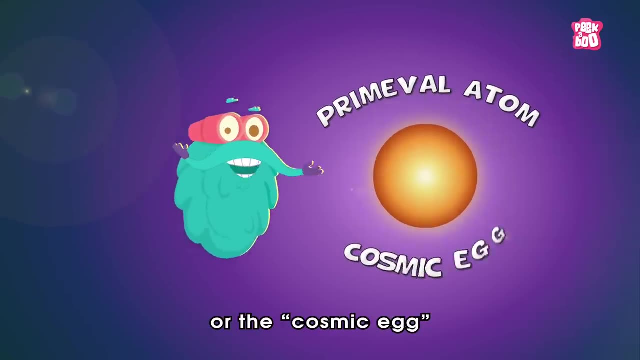 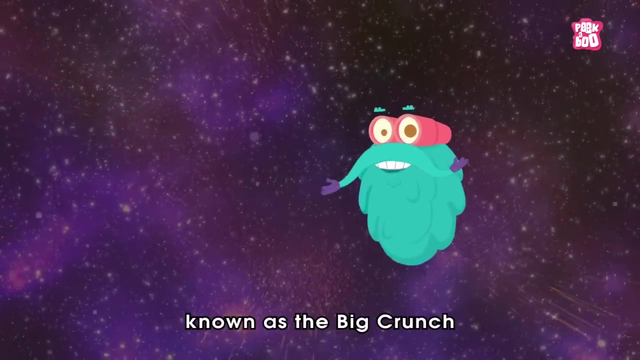 The single super concentrated point or bubble, which later became the universe before the big bang, was called the primeval atom or the cosmic egg. Also, in one of the possible scenarios for the ultimate fate of the universe known as the big crunch, the universe will eventually stop expanding. 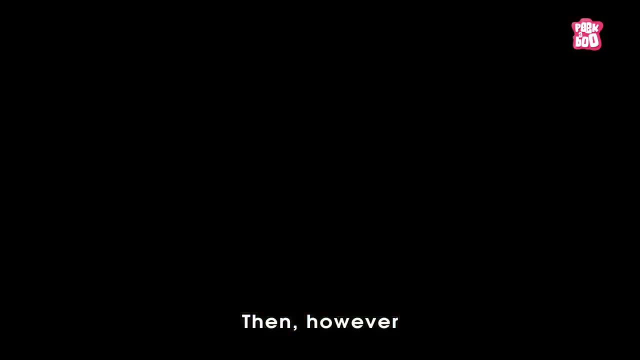 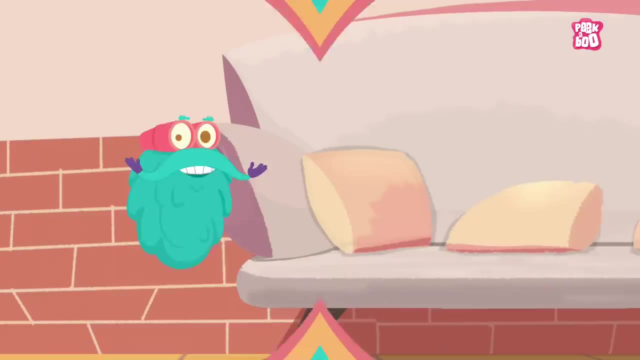 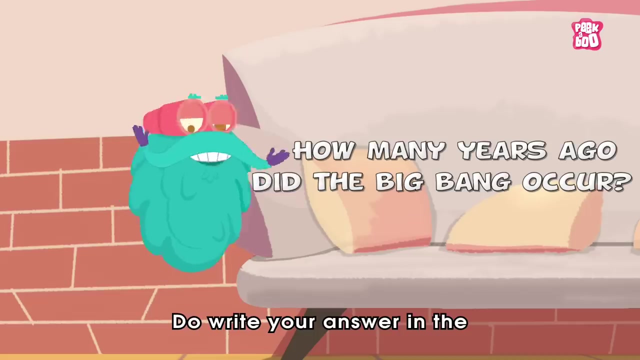 and start collapsing in on itself. Then, however, another big bang might happen. It's question time. Today's question is: how many years ago did the big bang occur? Do write your answer in the comment section below and hit the like and subscribe button if you haven't yet.